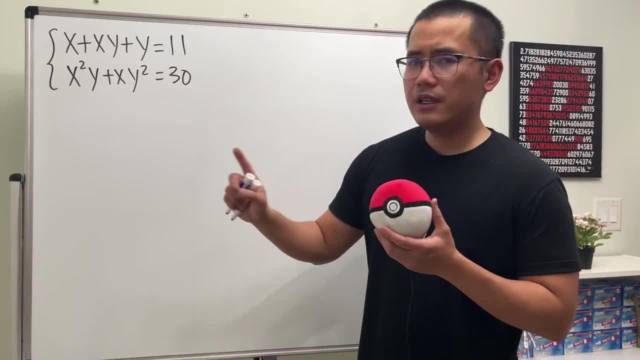 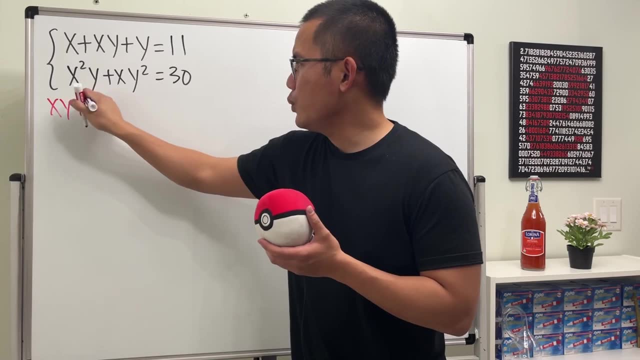 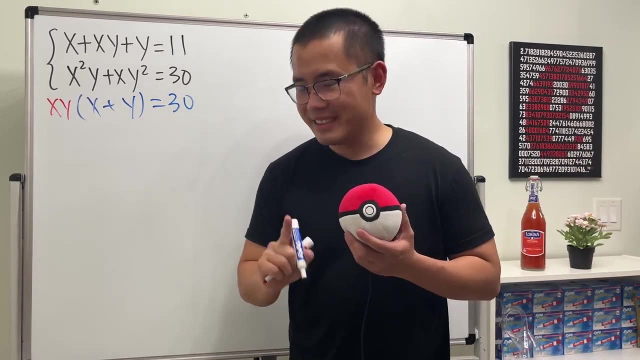 So let's see, I think it's a good idea to look at the second equation. We can do some factoring From here. let's factor out x, y, and then we will get x plus y and that will be equal to 30.. Ah, do you see it? You see that we have x, y. It's in the first equation. 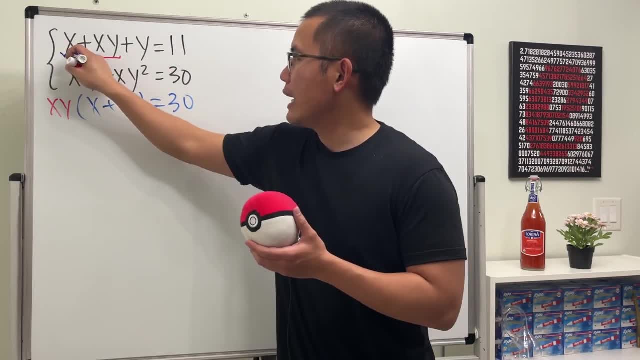 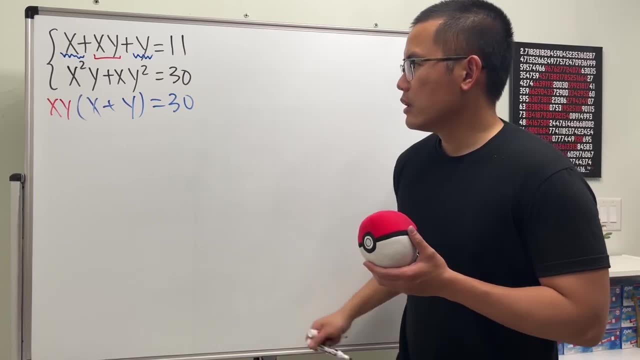 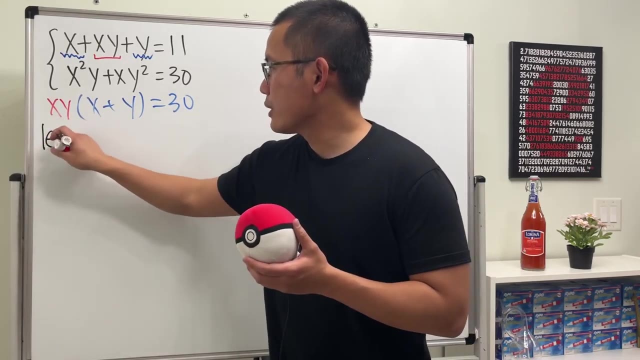 right here, and then x plus y we also have it right here. So what that means is that we can actually just do a very nice substitution. So instead of working with the x, y or x plus y, we're looking at this as a new variable, So I'm just going to code that to be: let's. 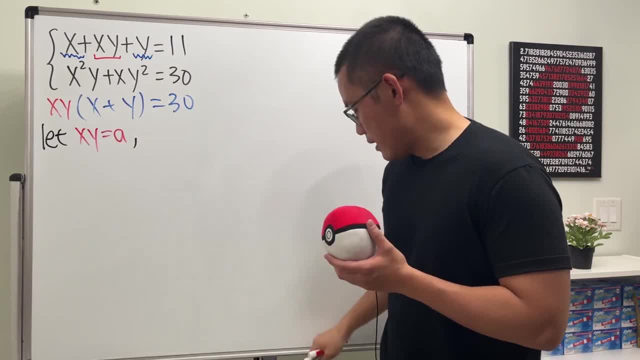 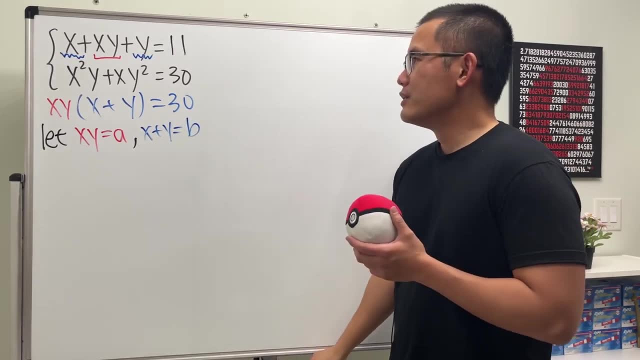 say a and then the other part right here, x plus y. let's code this to be no, not c, b. Yeah, just kidding. So if you take a look at these equations now, the first one can: 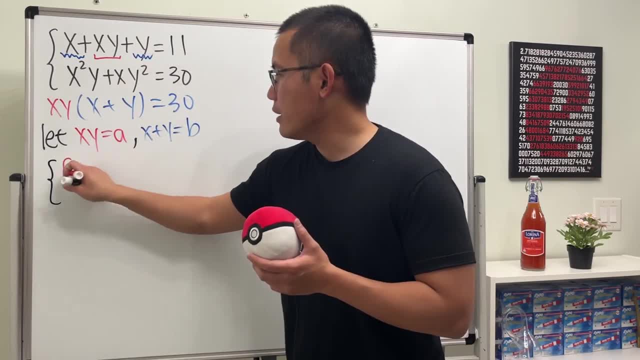 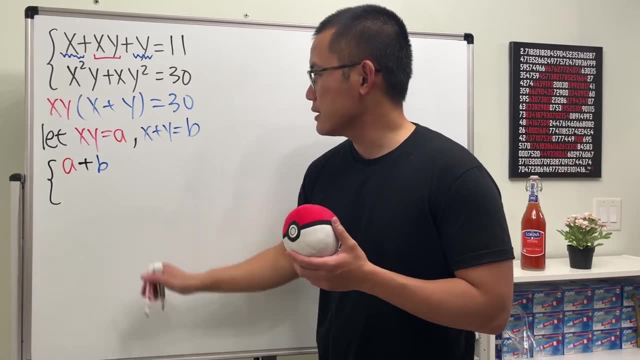 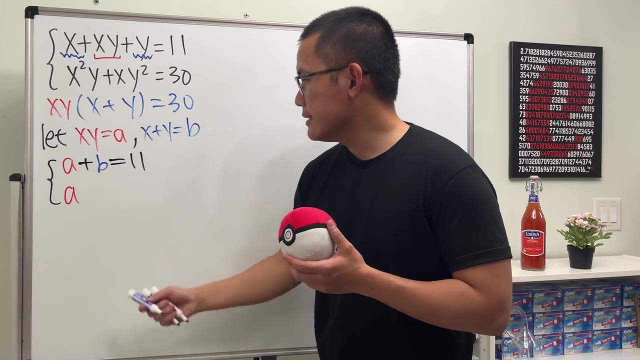 be written as We have the a right here, and then we just have to add this and that which is our b, and then that will be equal to 11.. so that's pretty nice. and then, secondly, we have the a and also the blue part, which is b, and this time it's. 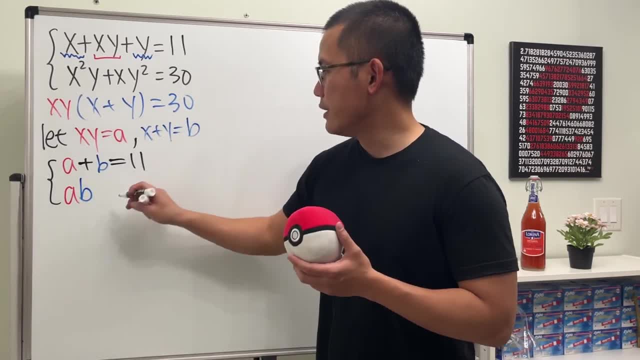 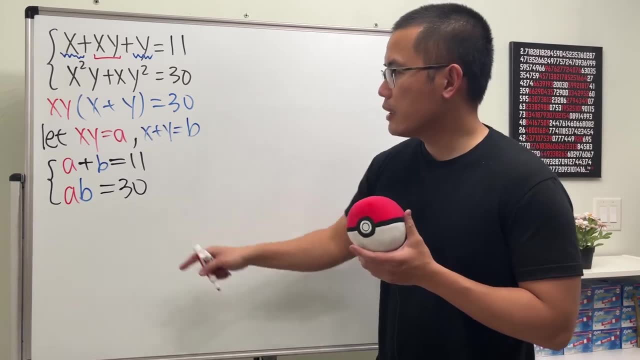 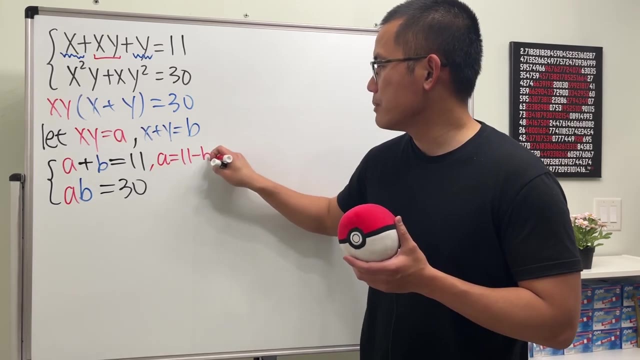 multiplication. so we have: a times b, it's equal to 30.. so now, this is much easier to work with and let's go ahead and proceed with a substitution. perhaps i will isolate the a, so i will move this to the other side. so this means a is equal to 11 minus b, and i'm just going to put this right here. 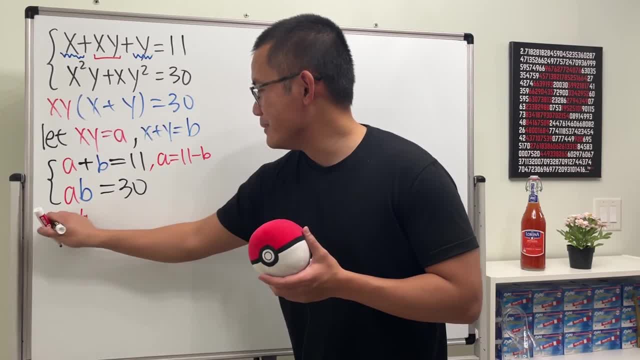 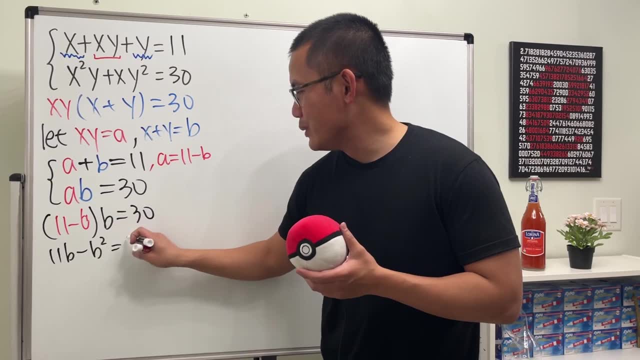 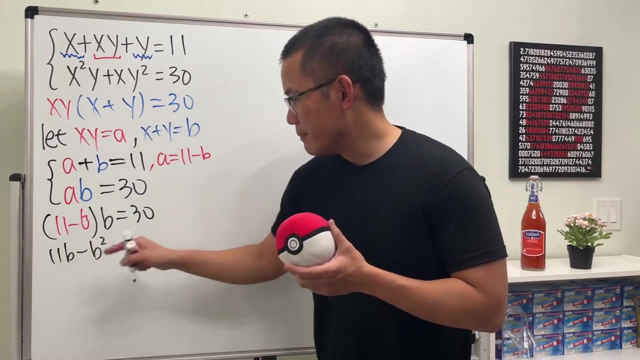 so we get 11 minus b times b is equal to 30. and then multiply things out. this is 11 b minus b, squared it's equal to 30. it's a quadratic right, just move things around. so this is going to let's- let's move these two terms to the other side, but i'm going to put that down first though. 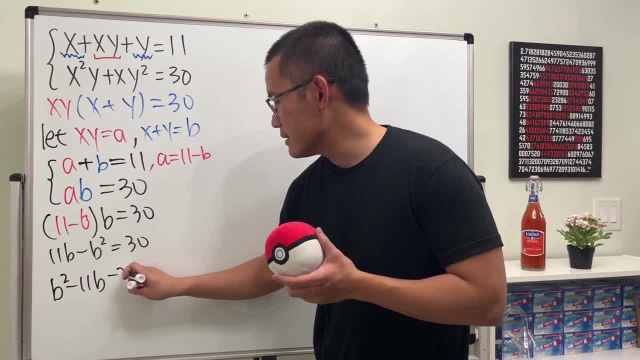 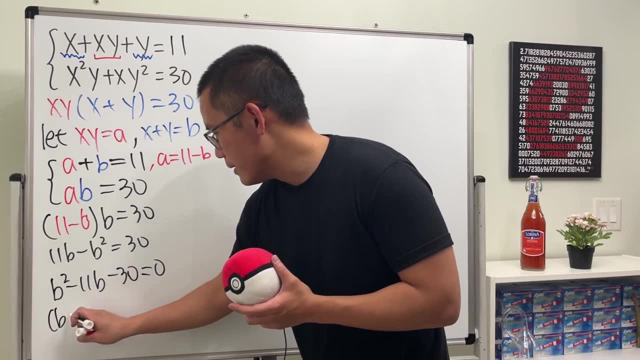 so b squared minus 11, b minus 30, is equal to 0, and then i will just solve this one for you guys by factoring. okay, so we have b minus 5. actually, no, it's plus positive 30, because i moved these two terms to the other side. so it's: 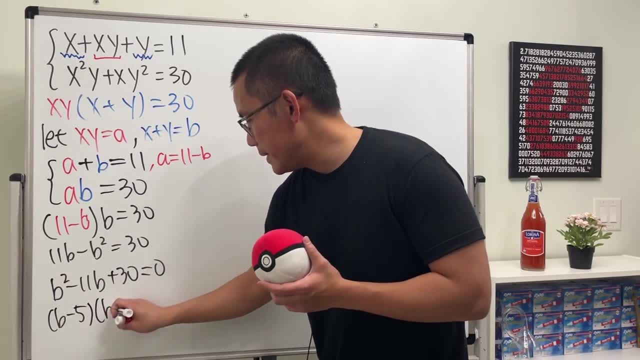 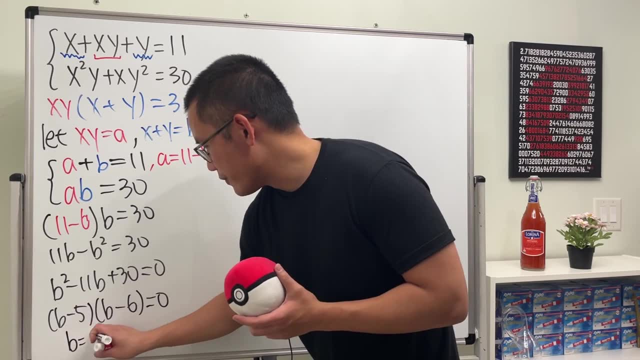 plus 30. so b minus 5 times b minus 6 is equal to 0.. so this means we have: either b is equal to 5 or b is equal to 6.. no, we're not done yet, don't be too happy. 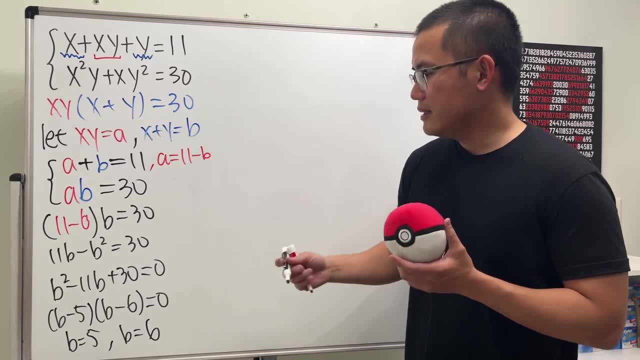 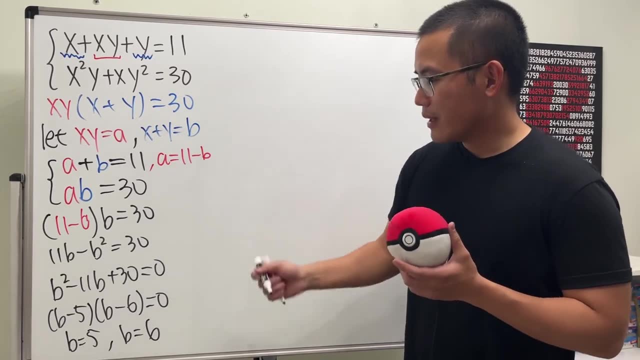 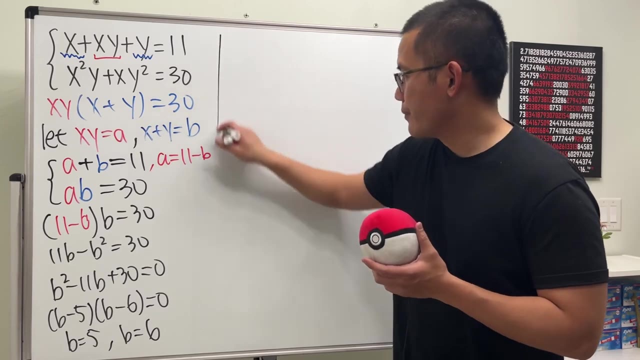 and you know what. we also have to figure out the a. and this is the bizarre part. we have a lot of combinations, or four of them to be exact, you'll see. but let's see. when b is equal to five, that means a is equal to. let's put it down here: when b is equal to 5, this means a is equal to. 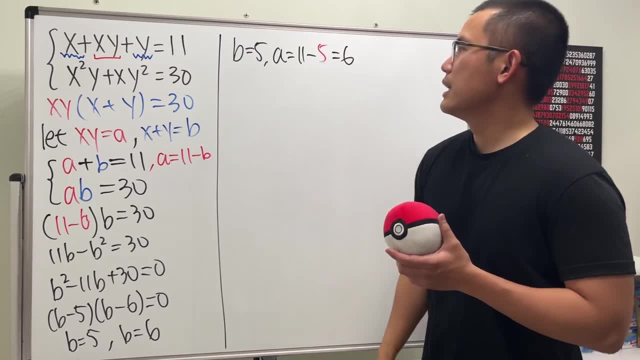 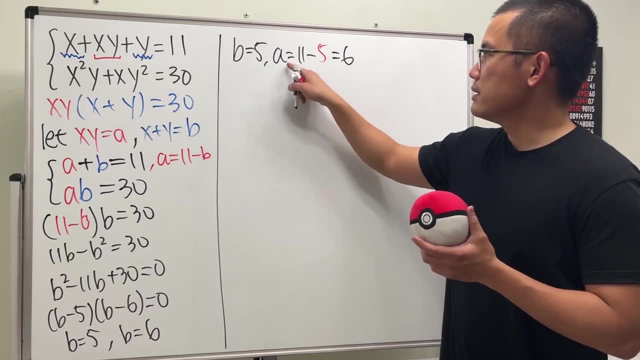 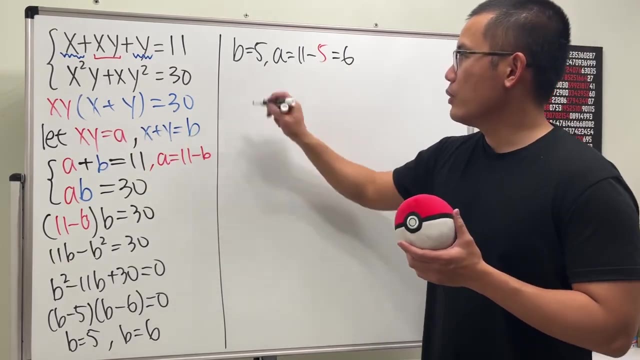 11 minus 5, which is 6.. and let's just focus on this one right here first. right, so this is like the first case, because what we have to do next is: b is equal to- sorry, a is equal to 6 and b is equal to 5.. we will have to set this back right here. so this means x times y is equal to the. 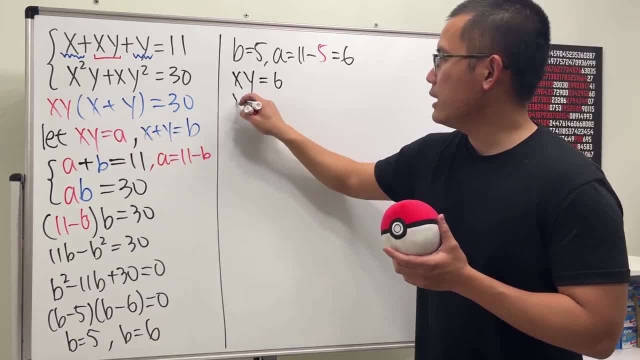 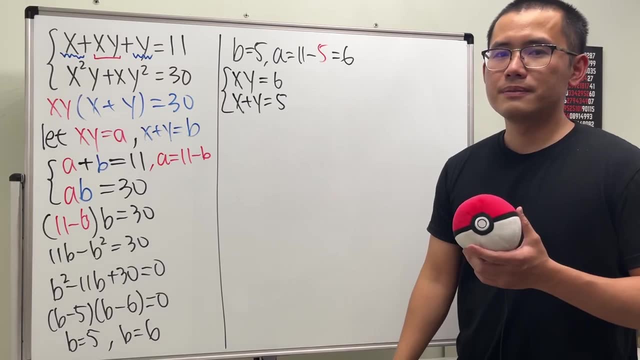 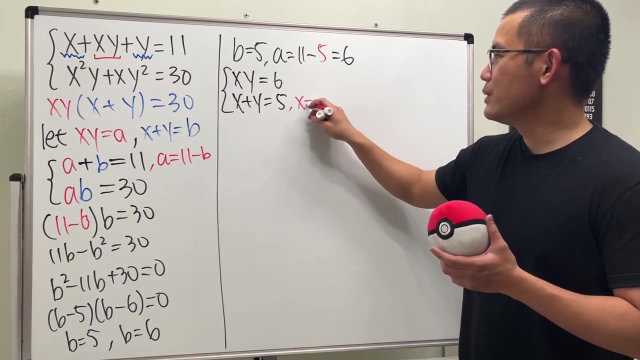 a value, which is 6, and then x plus y, which is equal to the b value, which is equal to 5.. oh yeah, another system of equations. do this by substitution again, so i'm just going to move the y to the other side. so this means x is equal to 5 minus y, and i'll put this back there, so we have 5 minus y. 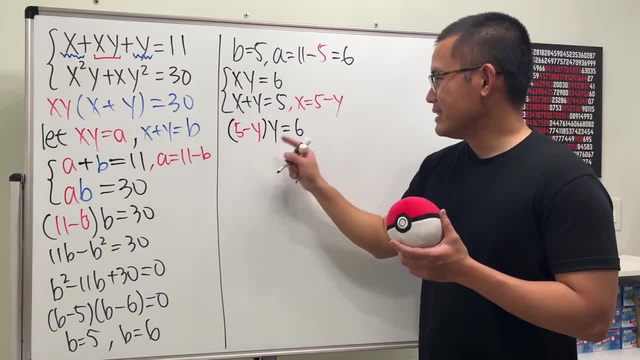 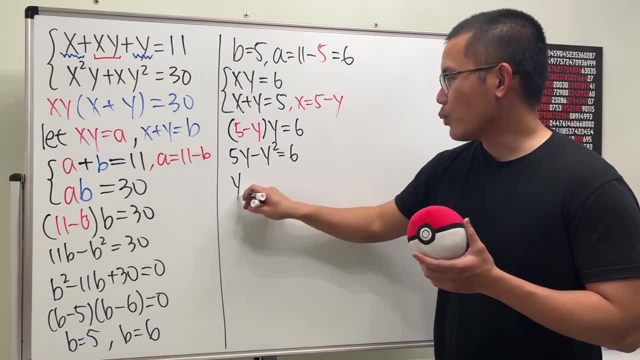 times y, it's equal to 6, and this is 5. y minus y squared is equal to 6.. move these two terms to the other side, but we'll write them down first. so y squared minus 5, y plus 6 is equal to 0. 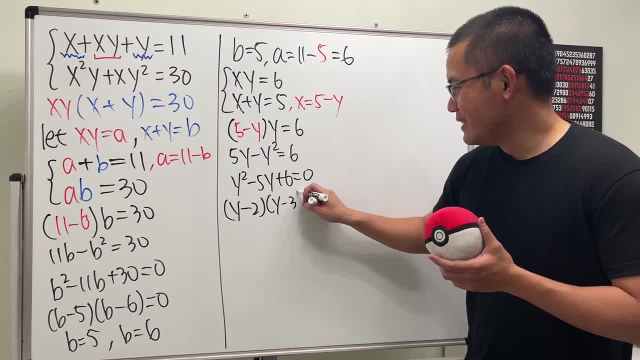 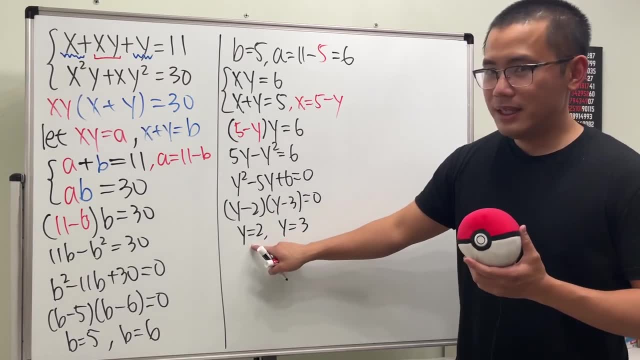 y minus 2 times y minus 3 is equal to 0. that means y is equal to 2 and the other one is equal to 2.. when y is equal to 2, x is equal to 5 minus y. so this right here tells us x is equal to five minus. 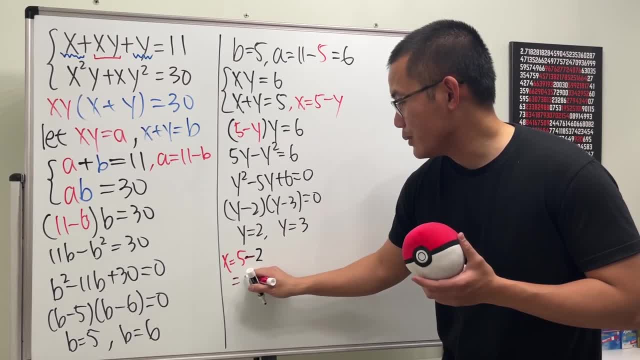 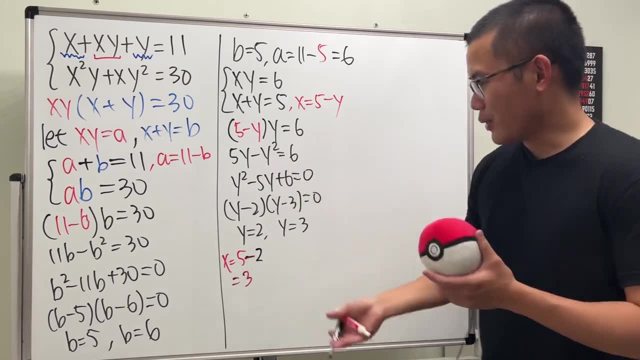 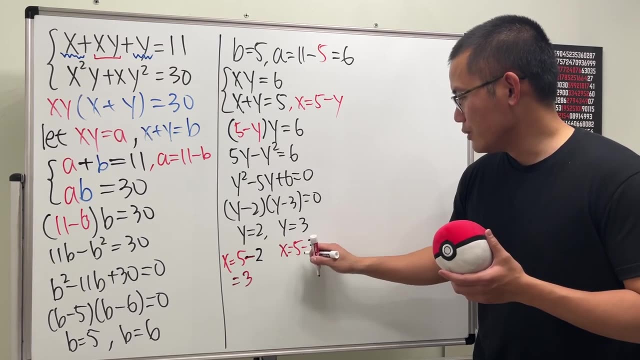 two. so that means x is equal to three. keep this in mind. it's crazy combinations, not like combination problem, but like the choice of the x and y. yeah, you know what i mean. and then the other one is: x equals 5 minus 3, which is equal to 2.. so we have 3, 1 minus x, which is 3. 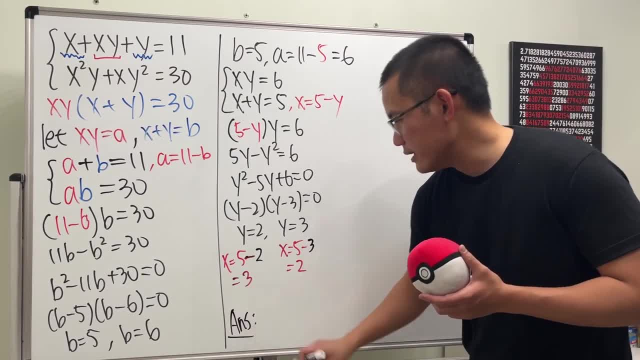 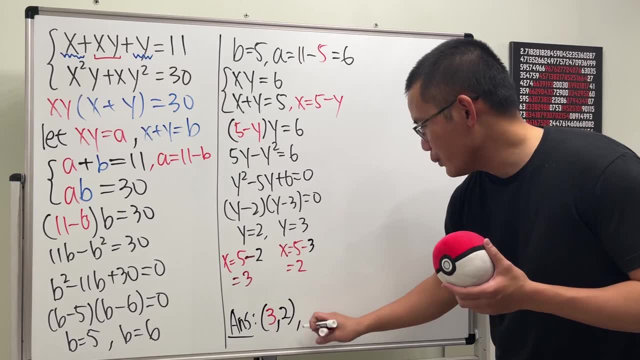 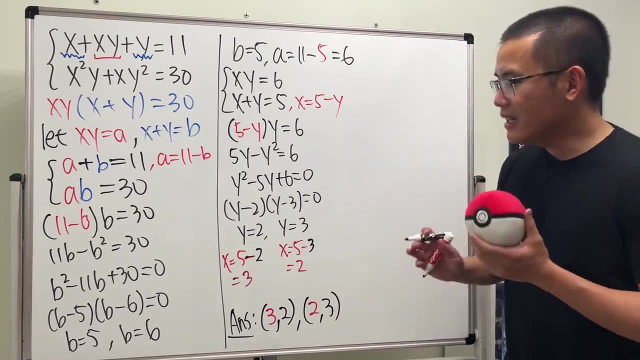 two answers so far. let me just put them down right here. answers: ladies and gentlemen, the first answer is three comma two. so just put on three in red and then two in black and then the other one's the opposite. so we have two comma three. right, and you think we're done? no, not yet, because remember we. 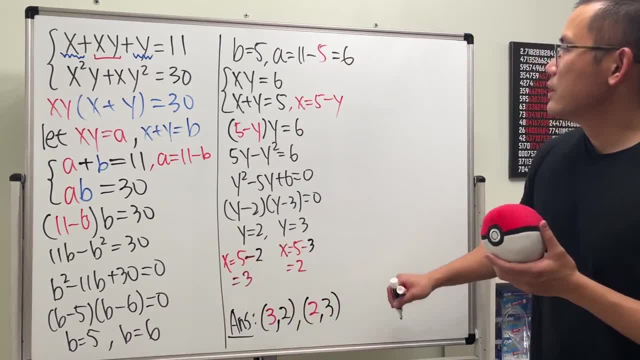 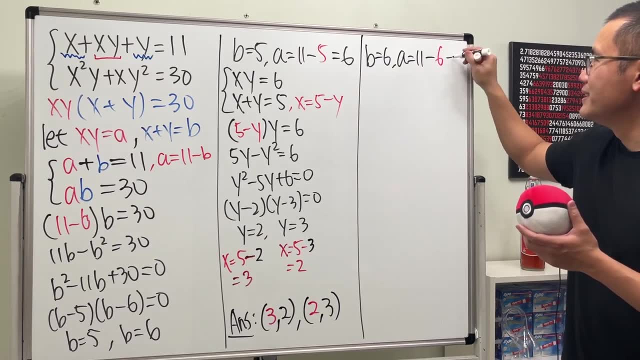 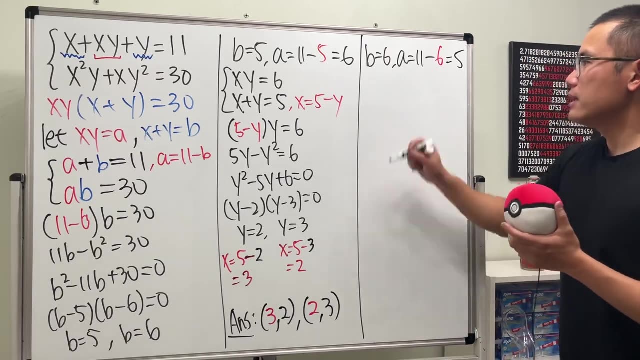 also have to look at this choice. when b is equal to six, so when b is equal to six, when b is equal to six, a is equal to eleven minus six, which is equal to five. yeah, this equation is very symmetrical, huh? yeah, by the way, let's go ahead and do it. so this means because a is equal to five, so 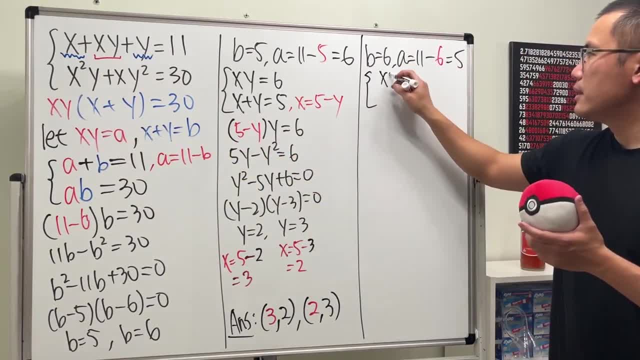 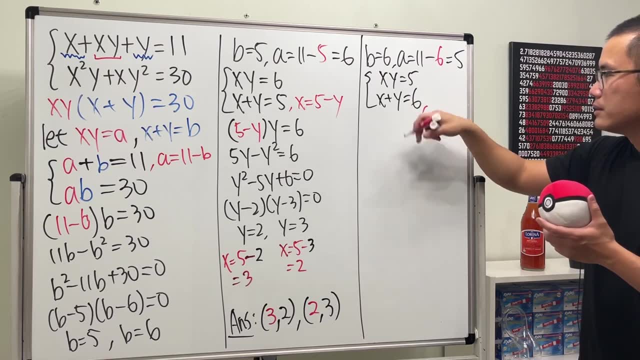 we have: x times y is equal to five. and then the other equation is: x plus y is equal to b, which is six, and then again i stop for the x right here. so that means x is equal to six minus y, and then put this right there. so we have six minus y times y is equal to five, and then just. 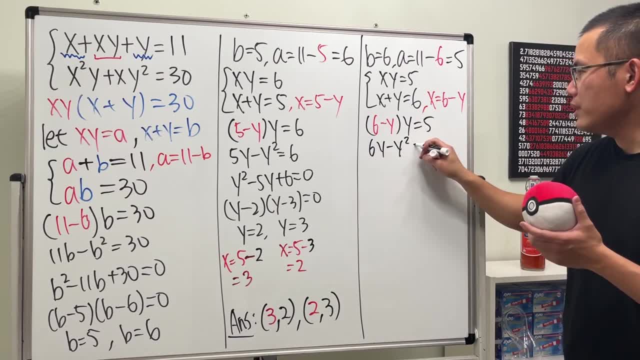 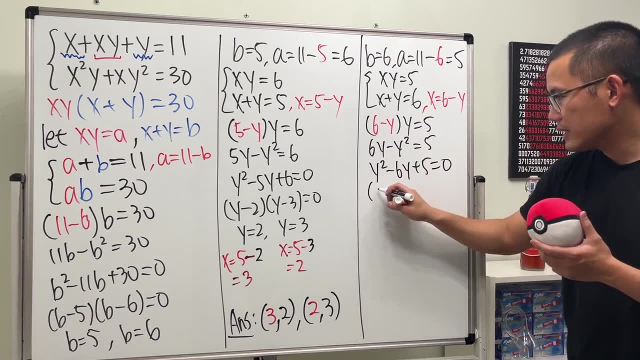 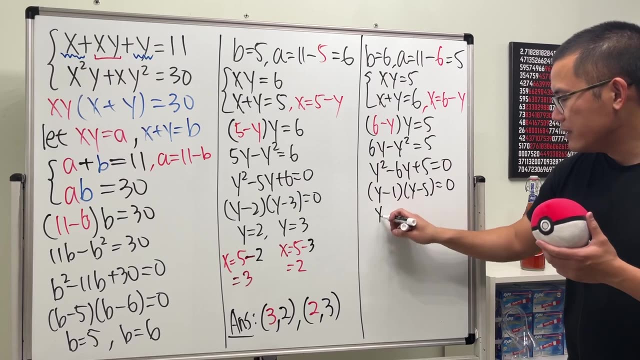 pretty much do the rest right. so this is six: y minus y squared is equal to five. y squared minus six, y plus five is equal to zero. and then this time we do y minus one, times y minus five is equal to zero. and we have: either y is equal to one or y is equal to five. when y is equal to one, 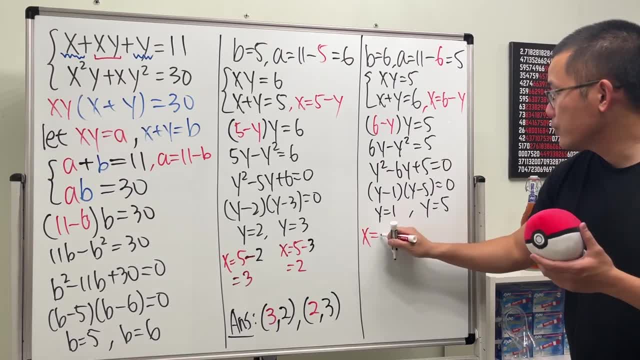 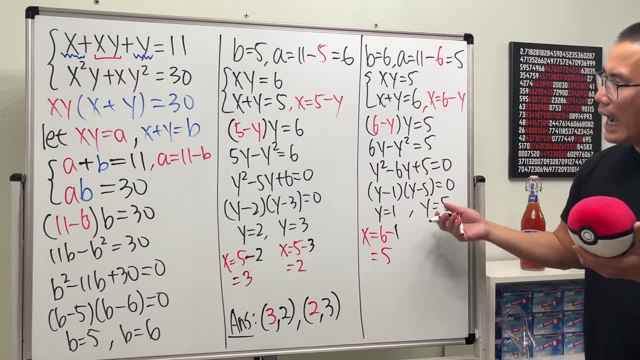 so we need to do the rest right. so we know that x is equal to six minus y, the other, like we know, it's going to be a four, and then we have minus one times y is equal to five. so we have y is equal to five and y is equal to zero, and then we have x and then we have a zero. so i don't. 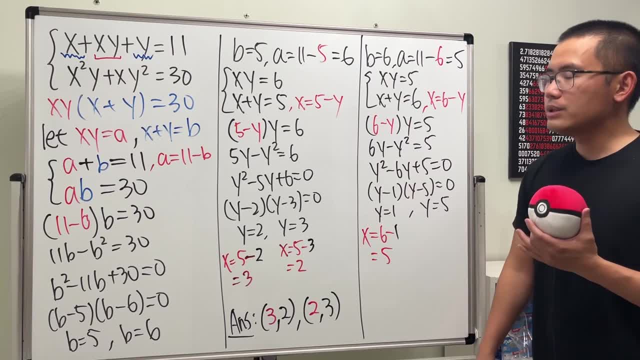 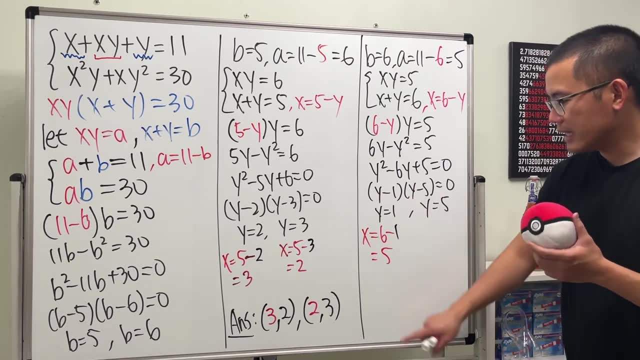 know how to do that right. so if we do it right here, we make it equal to y. this means y is equal to zero. and then we remove it and we put it back here. this means x is equal to six minus one, which is equal to five. and you know, the other one is just the opposite. i feel like this gonna be an easier. 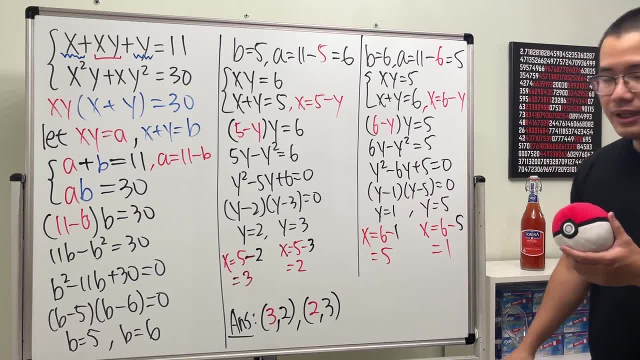 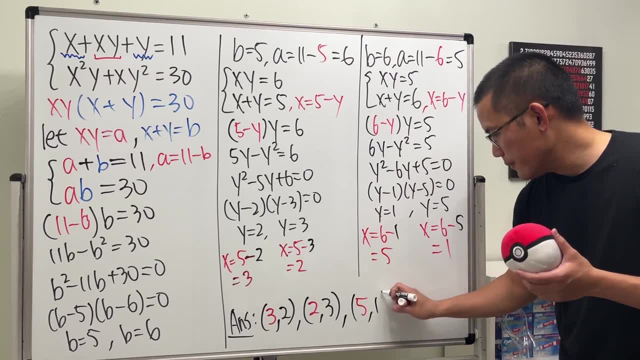 minus 5.. So that means x will be equal to 1.. So, ladies and gentlemen, two more solutions. The next one is 5 comma 1.. 5 comma 1.. And then, lastly, we have 1 comma 5..